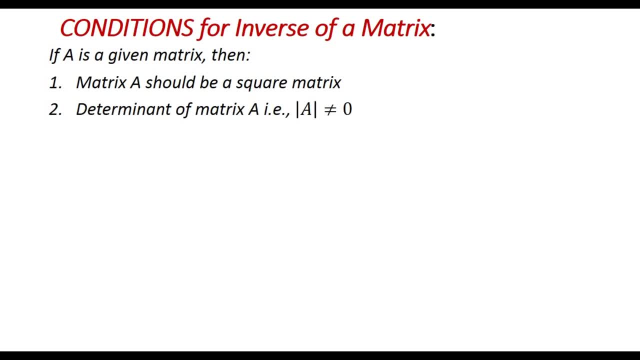 Which implies that it should be a non-singular matrix. Now, the first condition says that it should be a square matrix. So I hope you remember what is a square matrix. A square matrix is a matrix where the number of rows is equal to the number of columns. 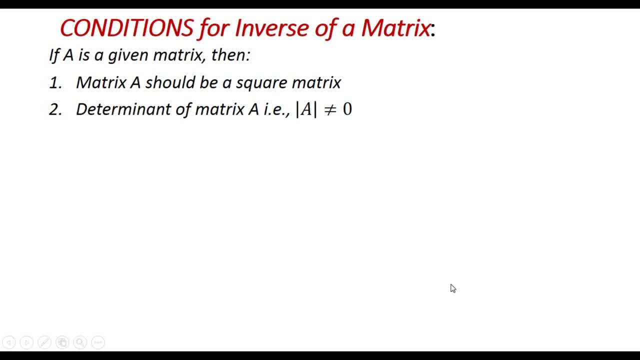 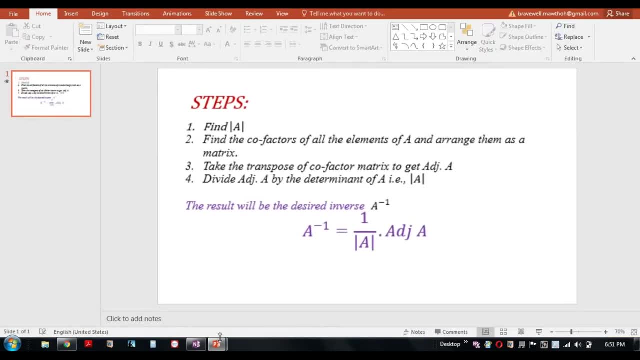 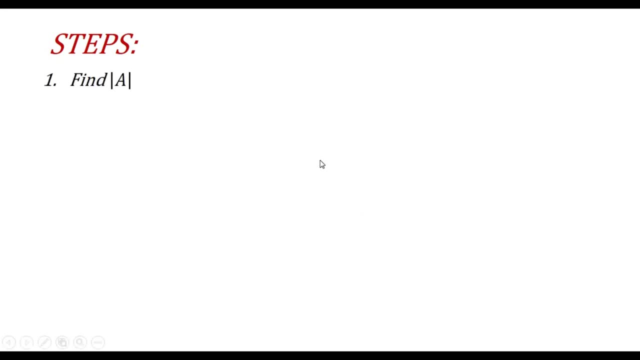 Now let us proceed and let us see what are the steps involved in finding the inverse of a matrix. The first step is to find the determinant of matrix A. So remember, if the determinant is equal to zero, Then it is not possible to find the inverse. 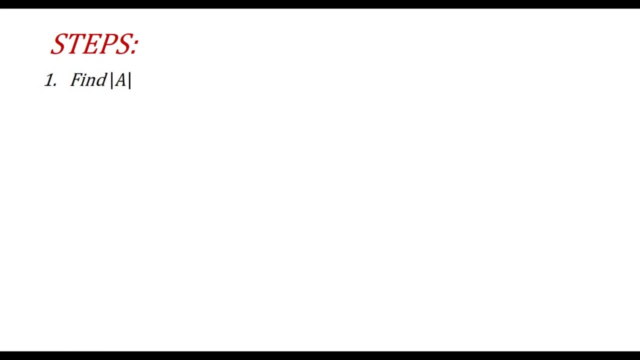 The inverse is not defined. We can only proceed if the determinant of matrix A is not equal to zero. That is, as I have mentioned earlier, it should be a non-singular matrix. The second step is that we need to find the cofactors of all elements of A and arrange. 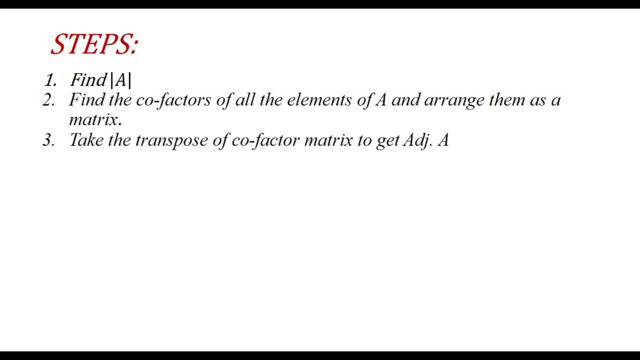 them as a matrix. The third step: we need to take the transpose of a cofactor matrix to get a joint A. What is the transpose of a cofactor matrix? If we take the transpose of any given matrix, then we interchange the rows into columns. 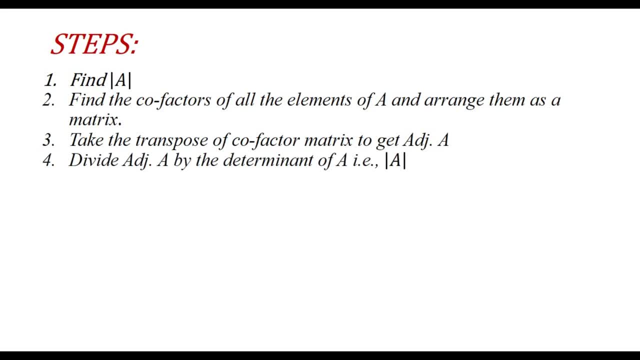 You shall see this later. The next step is that we need to divide a joint A, that is, a joint matrix of A, by the determinant of A. So the result will be the desired A inverse. Now here is again. the formula: A inverse is equal to 1 by determinant A at joint A. 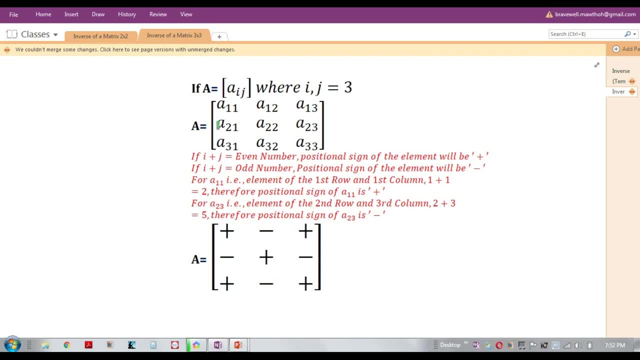 So let us see how the positional sign of an element is determined. So out here I am taking a square matrix of 3 by 3 order. So A is equal to Aij, where i is the number of rows equal to 3, and now j is the number. 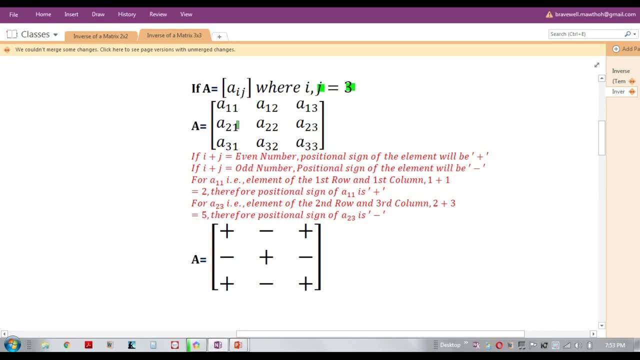 of columns. This is also equal to j. So j is the number of rows, equal to 3, and now j is the number of columns. This is also equal to j. So the first element- A11,, shows that it is present in the first row and first column. 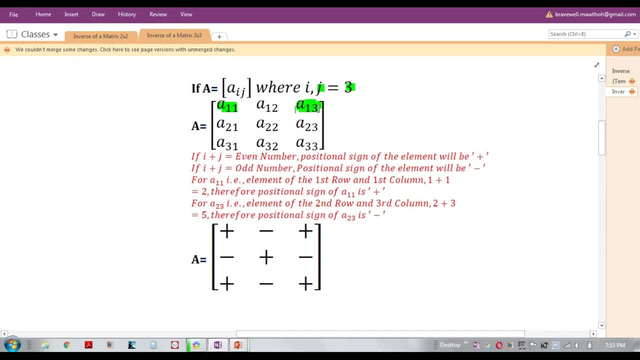 If we look at this element, this shows that it is present in the first row and third column. Suppose: if we look at this element, then it implies that j is the number of rows equal to j. It implies that j is present in the third row and first column. 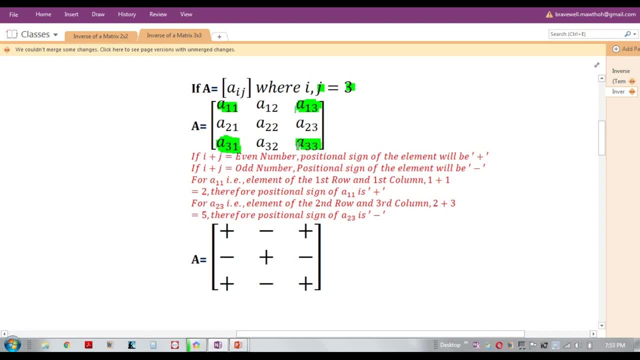 Similarly, if we look at this particular element, we see that j is present in the third row and third column. Now, how do we determine the positional sign of each element? Now, i is the row where j is the number of rows equal to j. 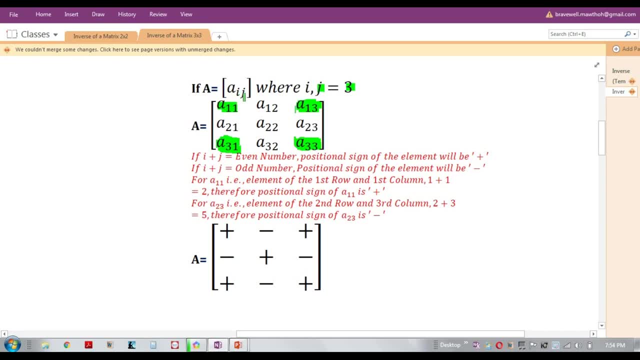 And i is the number of rows equal to j. element is present and j is the column where the element is present. so if the sum of i plus j is equal to an even number, then the positional sign of the element will be positive. however, if the sum of i plus j is equal to an odd, 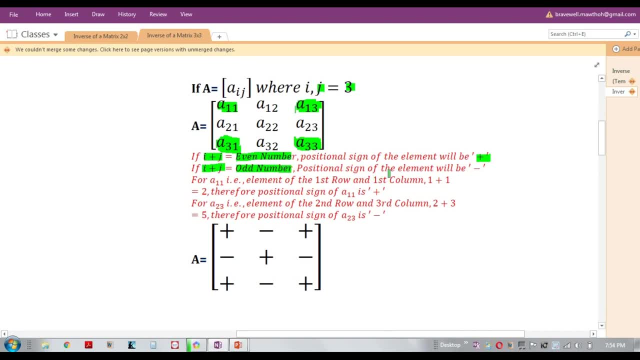 number, then the positional sign of the element will be minus. let us take an example of a 1: 1, so a 1: 1. this particular element is present, the first row and first column. so 1 plus 1 is equal to 2, so it is an even number. so